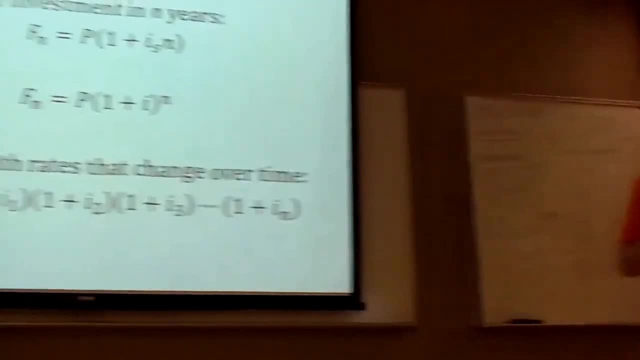 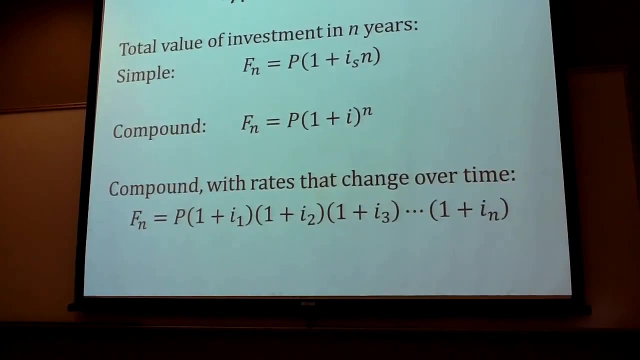 So there's two types of interest. You have simple and compound. And simple interest is just a period over time. But compound interest means that you're making interest on the interest. 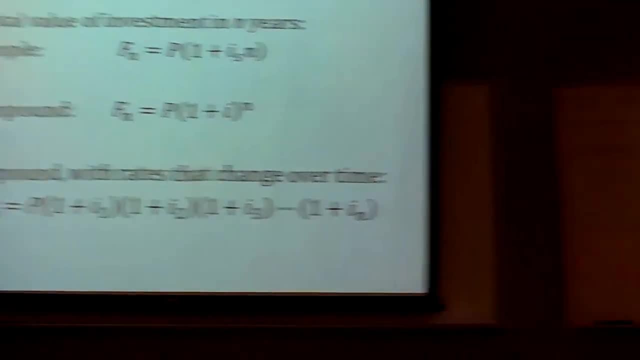 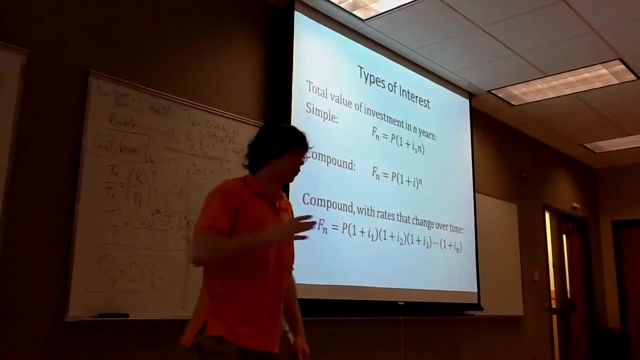 So if you have a certain amount of if you have an investment, you're not only making interest off of your initial investment, but you're also making interest off the interest. And interest is a cure year after year after year. 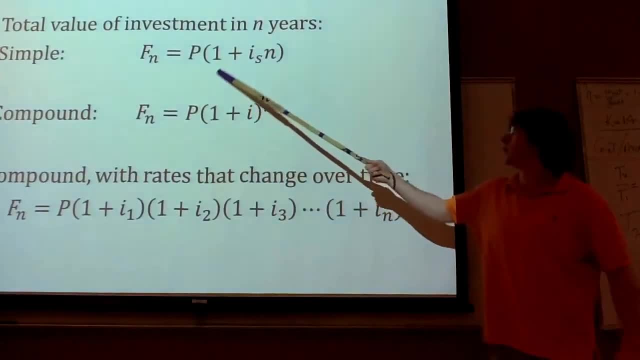 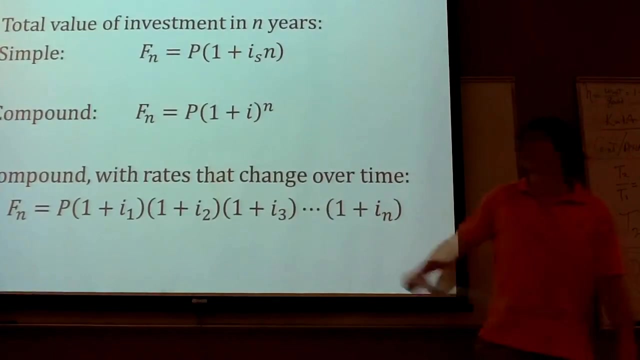 So the basic is just your interest times your number of years plus one. So that'll give you a decimal place, 1.07. Times your price is the value. So in this, S is your value and P is your price. 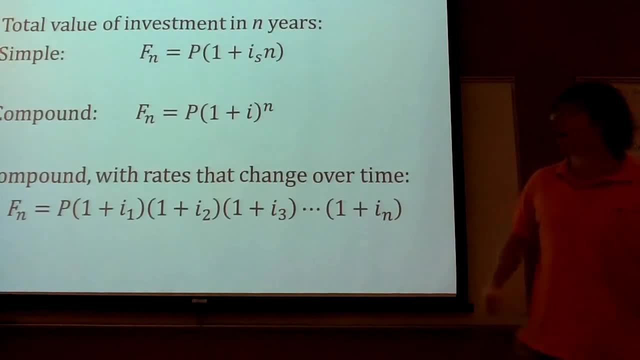 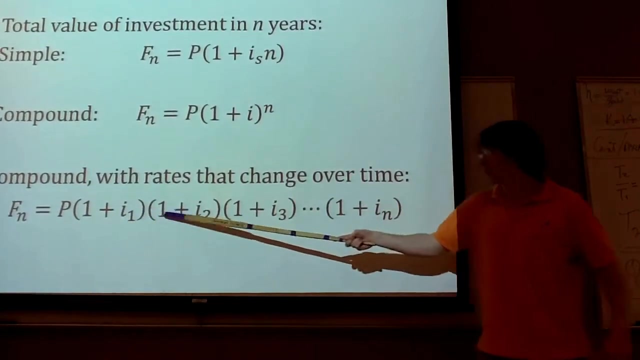 So P is the actual money and F is what your money is worth. And here, when you compound, what you're doing is you're taking your interest plus one, and then you're taking it to the number of times that it occurs. So, basically what you're doing is this down here. You're doing your price times one plus this, times one plus this, times one plus the interest, all the way out. 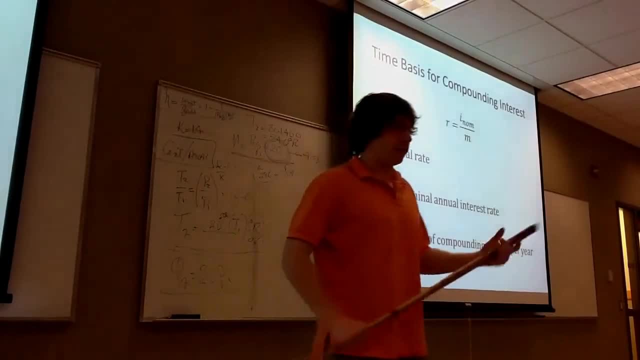 So the basic way to figure out your time basis for compound and interest, interest is your nominal rate of interest over the number of years that it compounds. 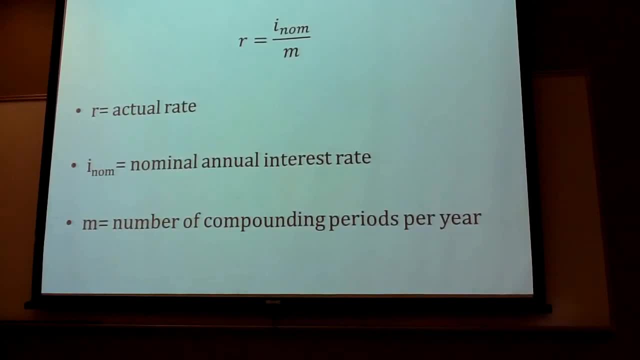 So that's a way to kind of simplify it into your actual rate that it compounds. 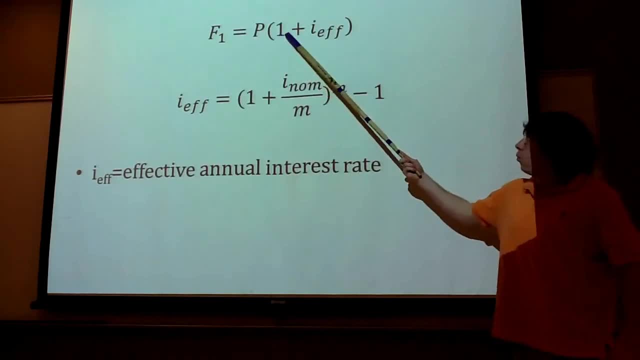 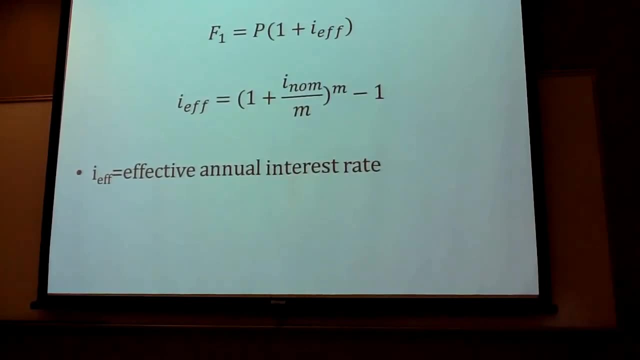 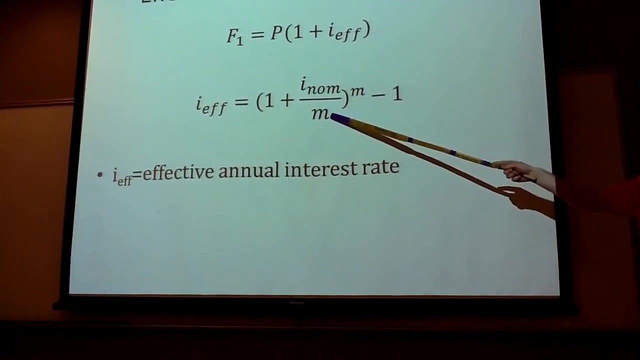 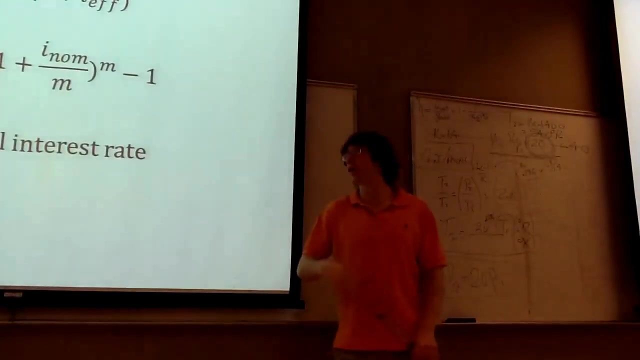 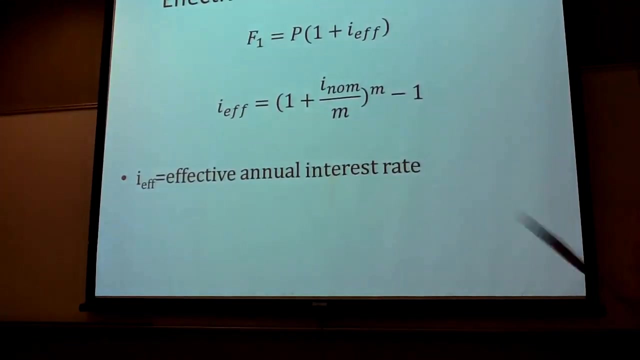 So the easiest way to see this is 1 plus your effective interest rate times the price will give you the value of your money, the future value of your money. And to go between nominal and effective interest rates, it's just kind of based off how often it accrues. So you just divide it by how often, the number of times that it accrues, whether it compounds quarterly, yearly, monthly. So you divide it by the number of times that it accrues, plus 1, so that'll give you a decimal, then you take it for power, and then you minus that 1. 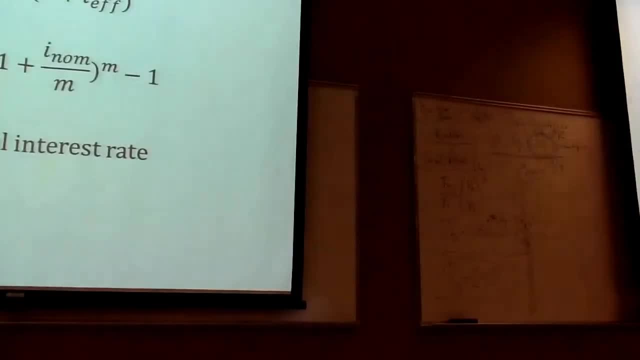 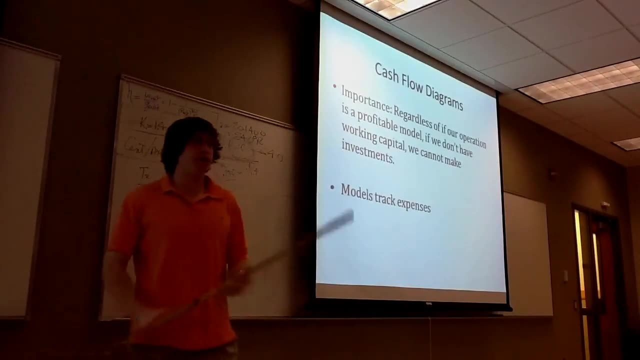 Now another big part of evaluating the profitability of an operation is a cash flow diagram. 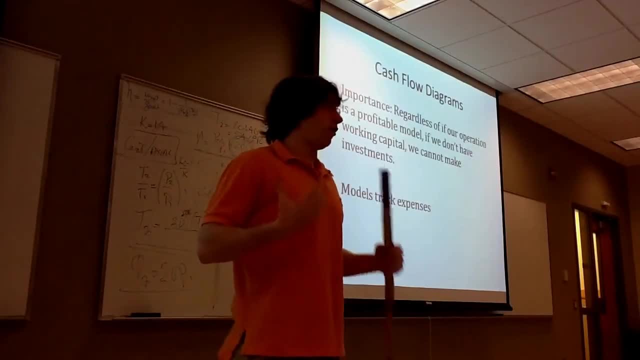 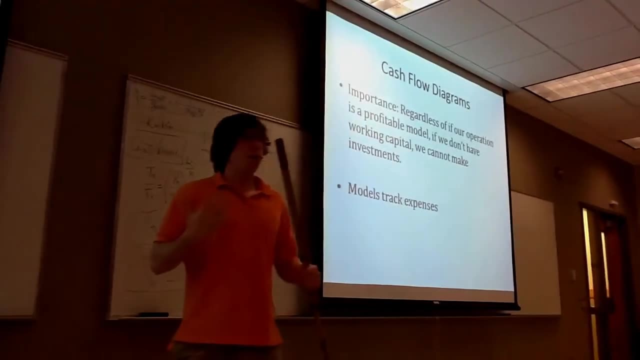 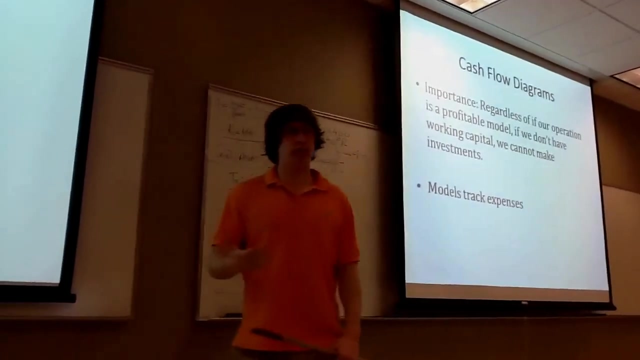 A cash flow diagram is very important because regardless of if our operation is a profitable model, if we don't have the cash flow to sustain our business model, we're not going to make, if we don't have any working capital, we can't make 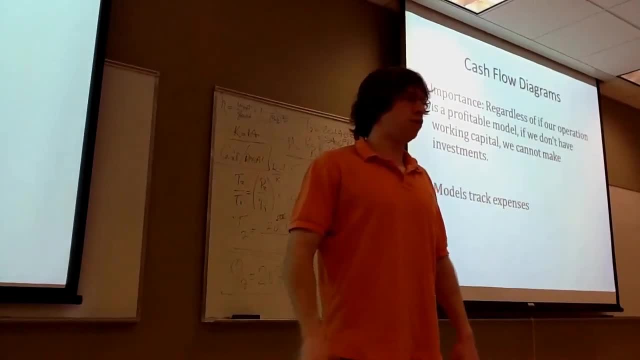 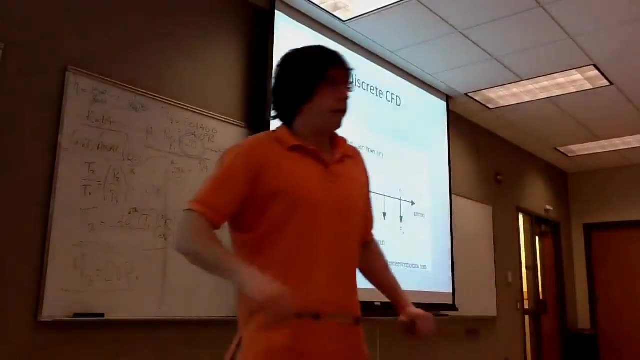 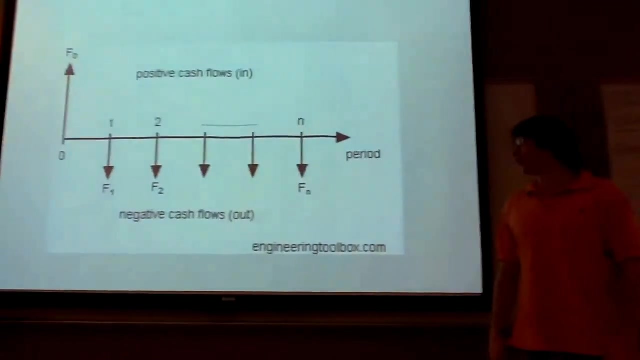 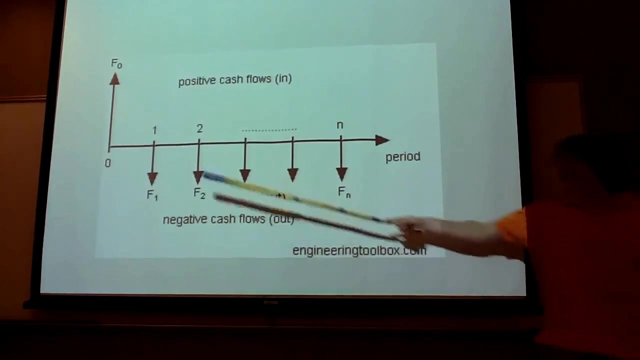 our investments in the project. So we've got to have models to track our expenses to make sure that we have cash in the bank to fund our investments. And the first one is a screep, and a screep just takes isolated expenditures and kind of gauges them against one another. You go up with anything, any cash coming in, you go up and down with any cash going out. So your credits and debits go up and down. And you just kind of come out like this. 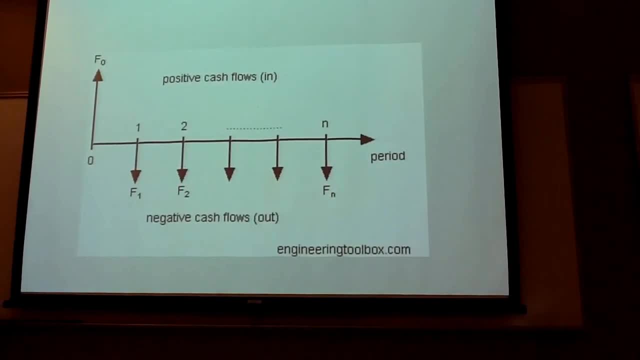 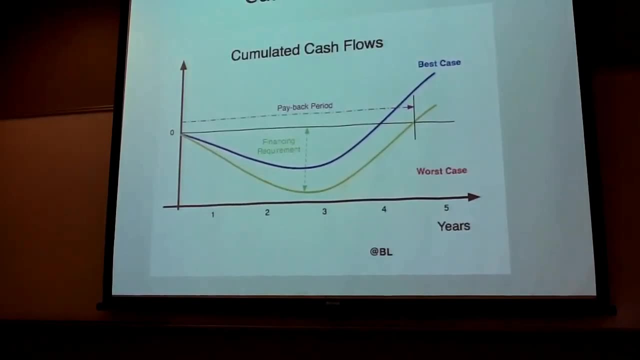 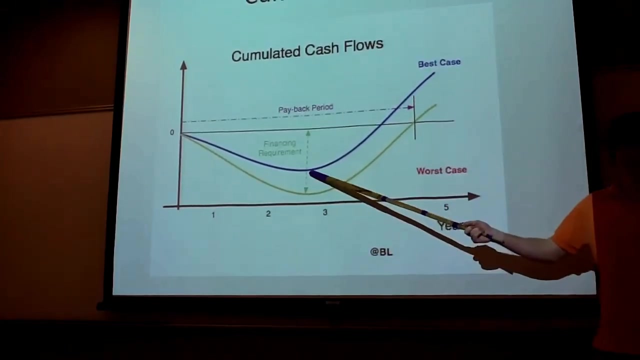 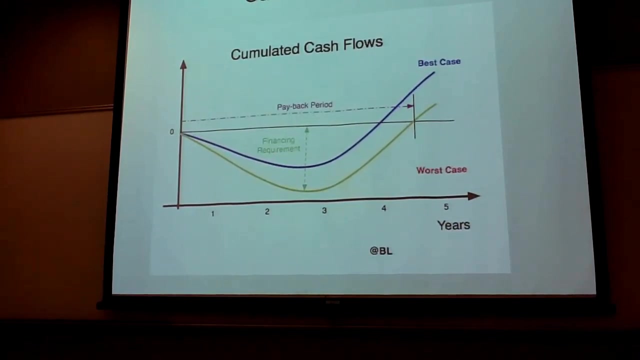 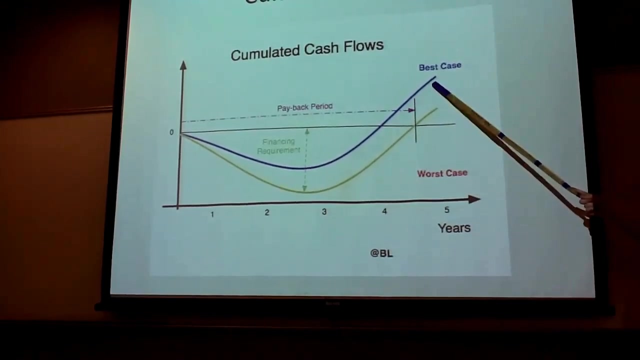 And then you can have a little chart over a period of time with how much money you've spent. And from that you can make a cumulative cash flow diagram. And a cumulative cash flow diagram kind of takes all factors into account, how much money you have in the bank and how over time what happens. And what happens is you start at .0, time 0, and over time you're going to spend something. You're going to be spending a lot of money in the beginning of your project to, you know, As far as there's a lot of capital costs and you're going to be paying a lot of people and you're not going to be getting a lot of return off your project. Eventually, you're going to have lesser and lesser capital costs and your operating costs will stay the same, but hopefully you're making profits. So you'll eventually start to come up in a deposit and to be the black, as they say. 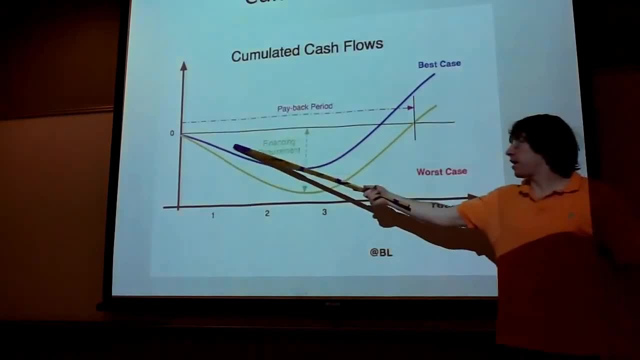 But the amount of time that it takes until you get from not making any money to making money, that's going to be your payback period. 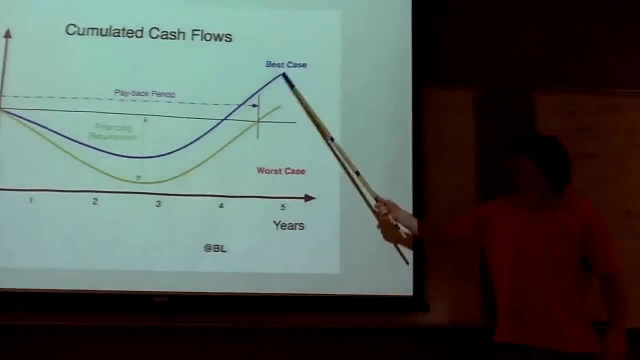 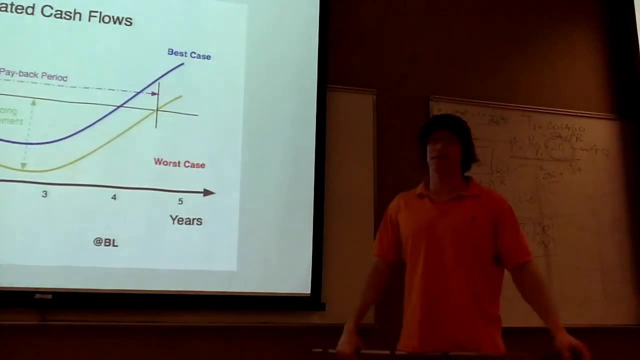 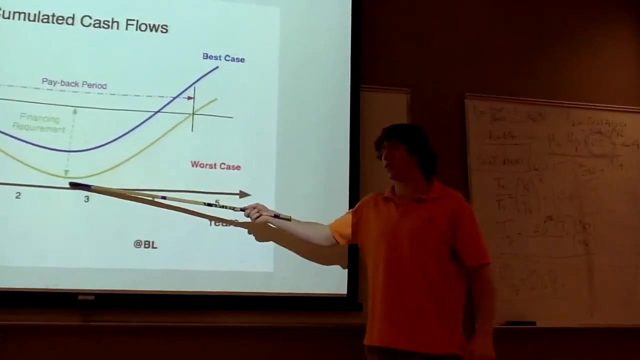 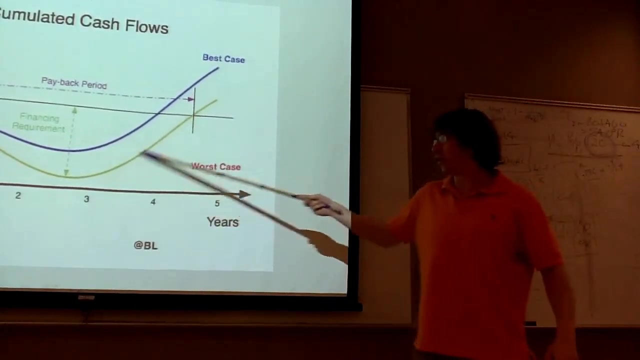 And what you want to do is you want to make a best-case scenario and a worst-case scenario. The best case being if everything goes perfectly, this is how much money you're going to spend. The worst case is if everything goes horribly, this is how much money you're going to be spending on the project. And your financing requirement is going to be as much as you're going to need, as low as possible. That's the point in the worst-case scenario because you've got to make it over the hump to when you start making a profit.